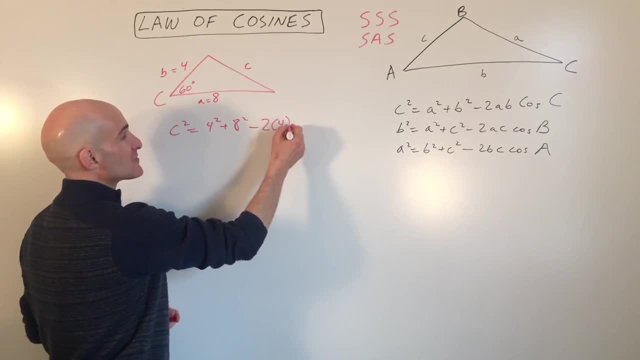 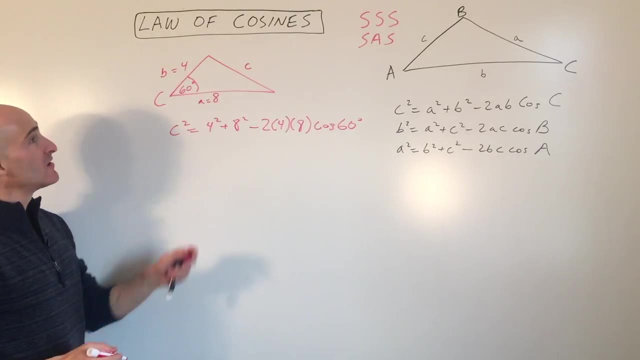 that angle minus 2 times, 4 times, 8 times the cosine of the included angle here: 60 degrees. So you can see, there's your side angle side and we're solving for the side across from angle C here, Here's side C, here's angle C. A and B are the two other sides that make up that angle. 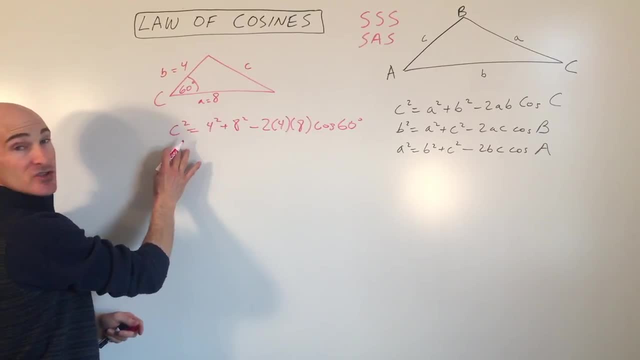 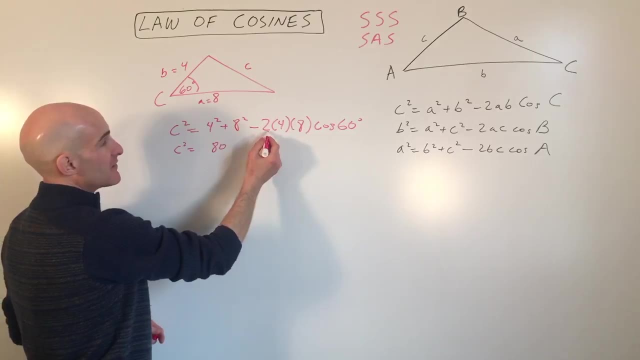 Okay, so all we have to do is solve this and then take the square root to solve for C. So what we have here, let's simplify: 16 plus 64 is 80.. Okay, and this is 2 times 4, is 8 times 8 is 64 times the. 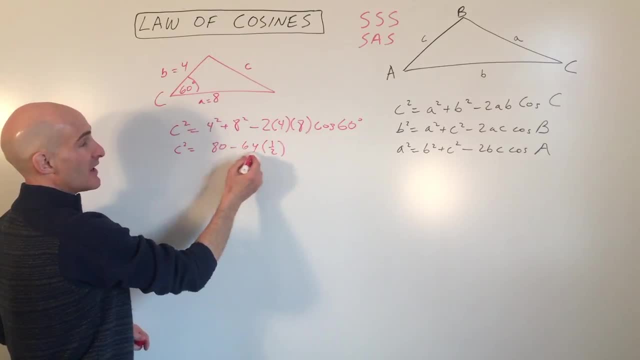 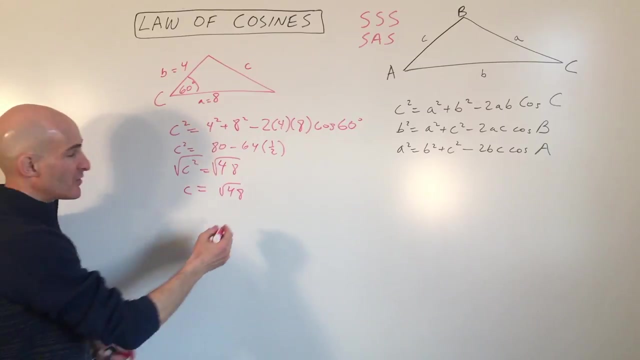 cosine of 60.. Cosine of 60 is a half, So we have 80 minus 32, which is 48.. Okay, and if we take the square root of both sides, we get the square root of 48.. And that's going to be the length of this side, And you can simplify this a little bit more. This is: 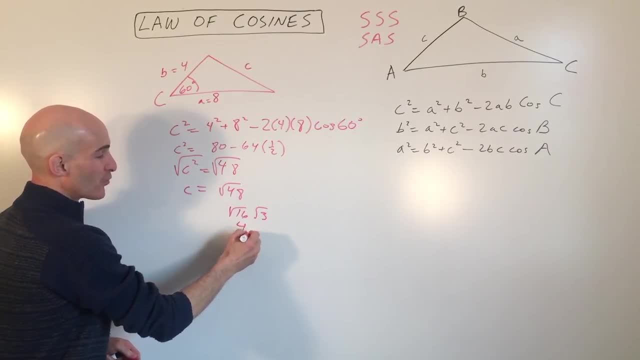 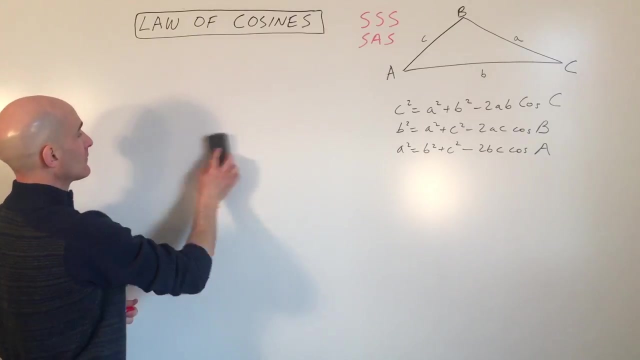 16 times 3,, which is 4 squared to 3.. Okay, so that's an example where you have side angle side. Let's do an example where they give you three sides. Okay, side, side side. So an example in this case would be something like this: Say: you're given 5,, 6,. 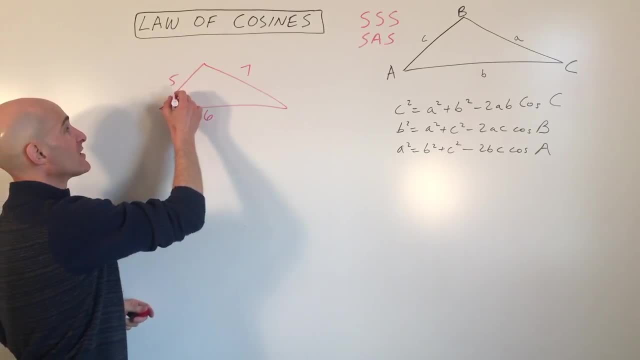 7. Okay, they're giving you just three sides And you want to solve for, let's say, this angle right here. We'll call it angle C again. So this would be side C, side A and B. Okay, so what we? 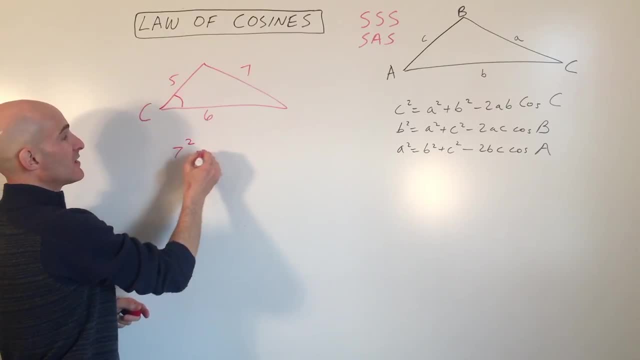 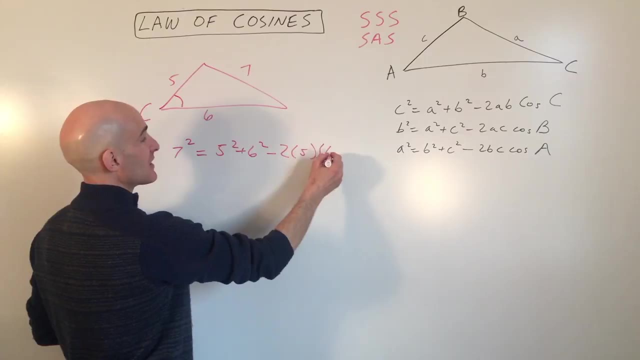 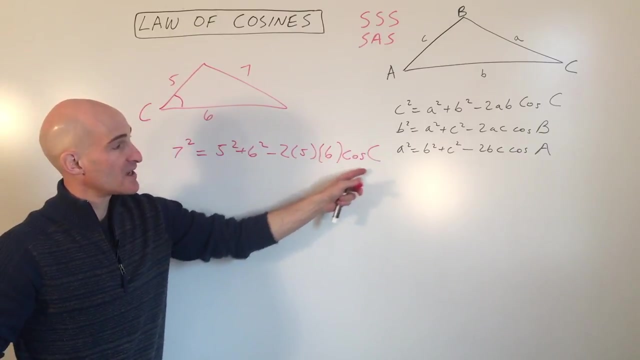 have here is: we have 7 squared. okay, equals 5 squared plus 6 squared, minus 2 times, 5 times 6 times the cosine of angle C. Okay, now what you want to do is you want to get this cosine C by. 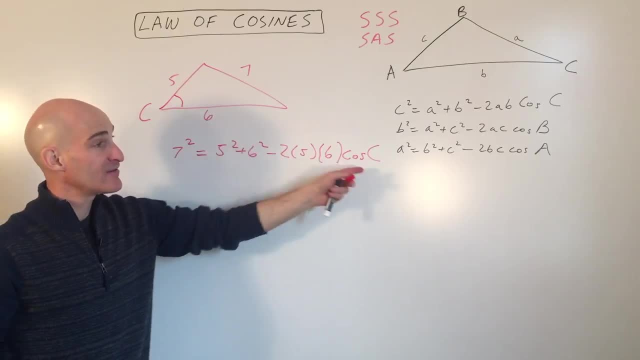 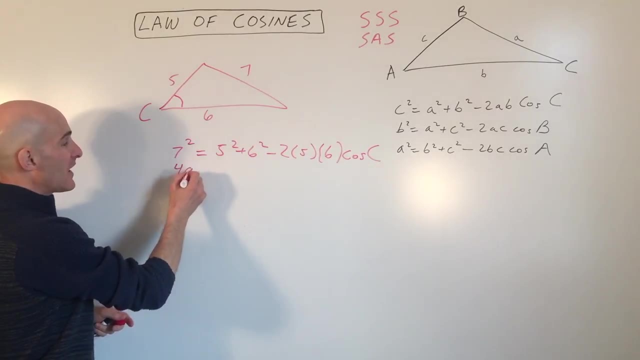 itself on one side of the equation. So you want to get this cosine C by itself on one side of the equation And then take the cosine inverse of both sides to solve for angle C. So what we're going to do is we're going to do this in steps. We have 49 equals 25 plus 36, which is 61,. 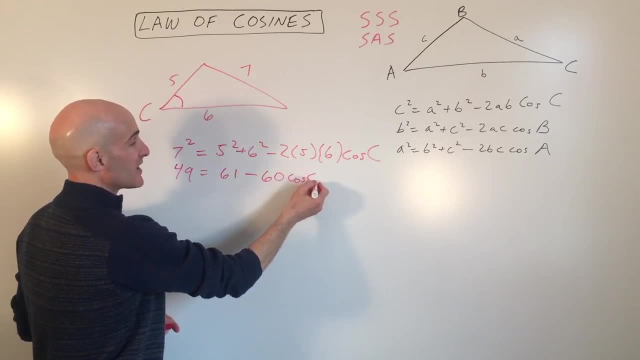 minus 60 cosine C. Now here's where some students make a mistake. They'll combine these and they'll say, oh, that's 1.. But you see, this is a group. These are all multiplied together. Okay, what you? 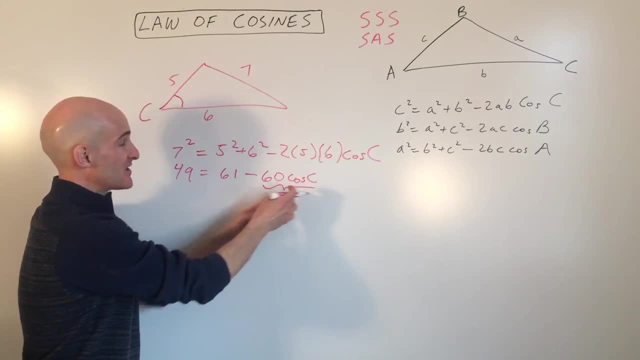 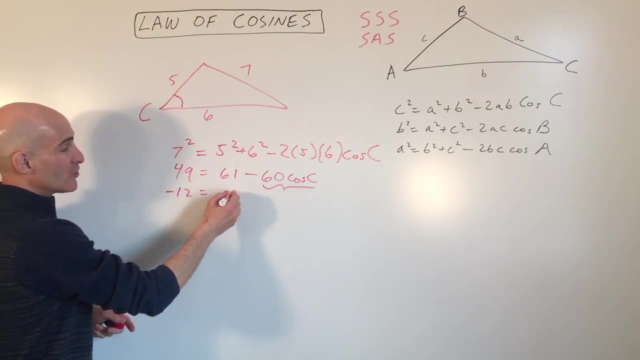 want to do is: you want to work from the outside in towards this cosine. So you want to work from the outside in towards this cosine to get it by itself. So I would subtract 61 from both sides, So that would give you negative 12 equals negative cosine C: negative, sorry, negative 60 cosine C. 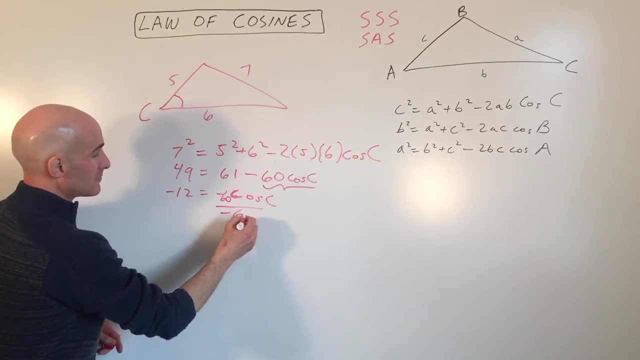 And then you divide both sides by negative 60, which equals cosine C, And that comes out to 1 fifth, which is 0.2.. And you take the cosine inverse of both sides, you're going to get C equals the cosine. 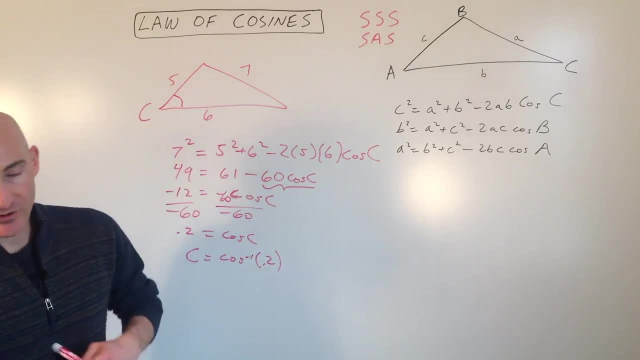 inverse of both sides, And that's going to give me 0.2.. And that's going to give me C equals migration inverse of 0.2.. So let's just see what that comes out to real quick here on our calculator. 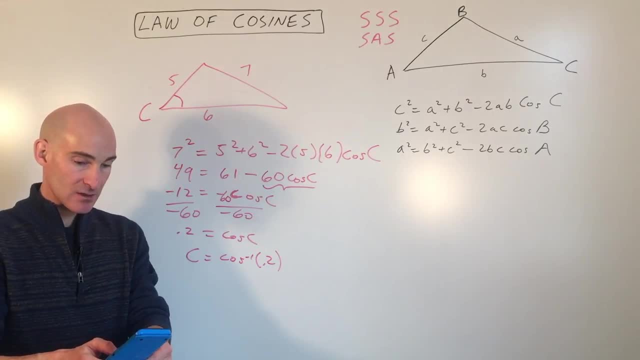 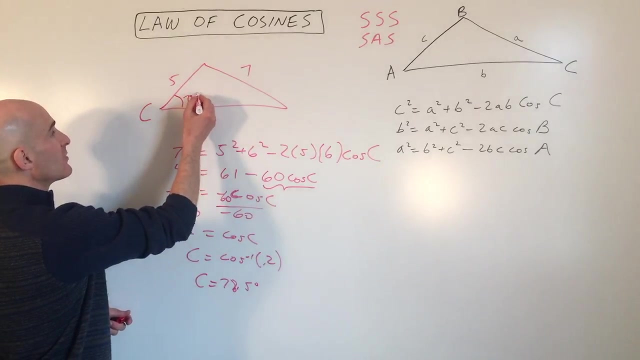 We have. let's see, we'll do it in degrees. Okay, degrees cosine inverse: 0.2, 78.5 degrees. So that's this angle right here: 78.5.. Now, if you want to solve for these other two angles, 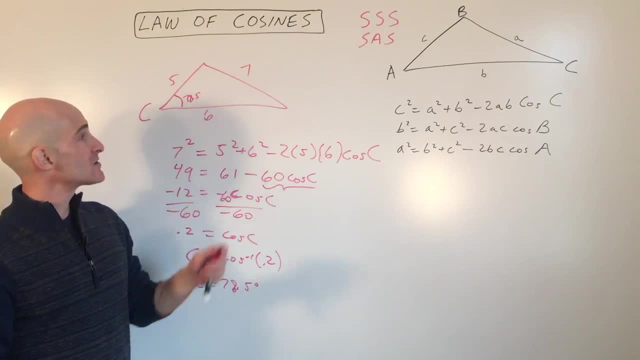 now you can use the law of sines. You only have to use the law of cosines at most. once You can use law of sines to find this angle, Then you have two angles. You can add those up and subtract from 180, and then you've solved the triangle. You found all the sides, all the angles.